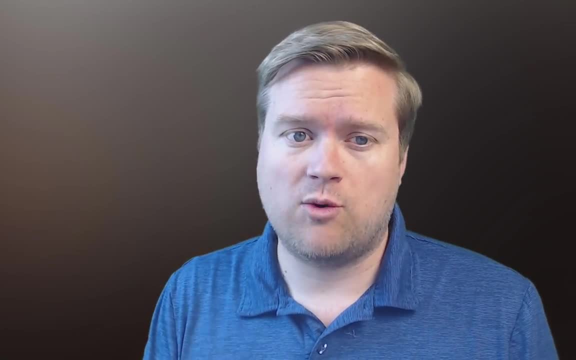 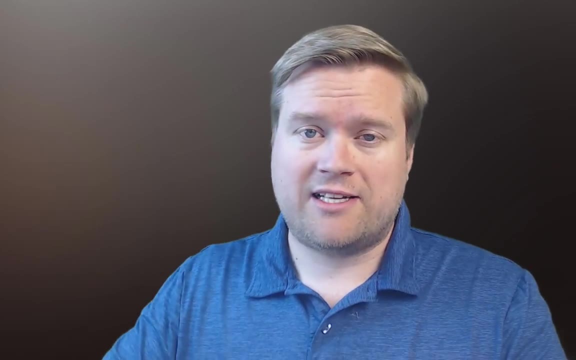 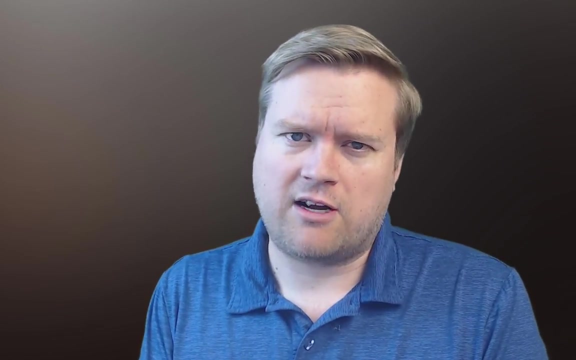 Hey, hey, developers. Today we're going to look at Element UI, which is a Vue 2.0 based component library for developers like you and me. So we are going to set up Element UI, We're going to kind of take a look at the different components that it offers and maybe kind of compare and 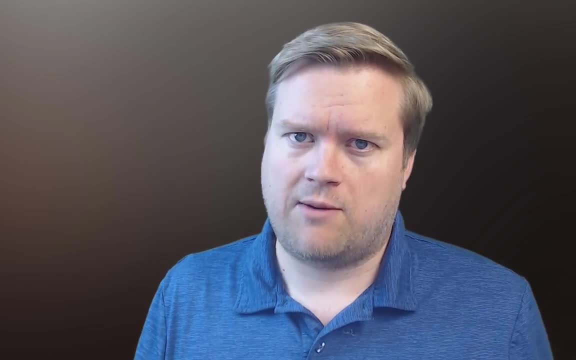 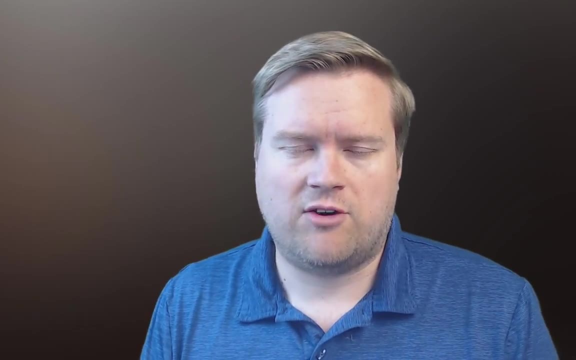 contrast that to other frameworks, other Vue component frameworks out there and talk about some of the differences. And one thing you might notice right away is that Element is really international focused. When you install it you can pick between Chinese, English and a bunch of 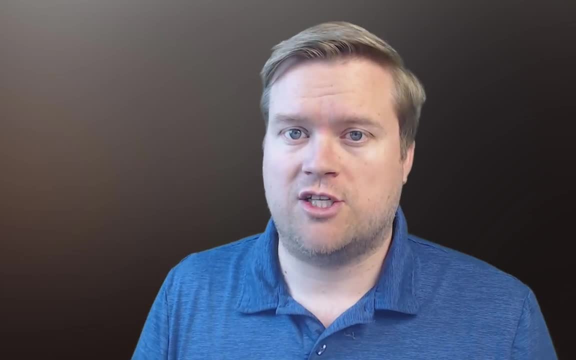 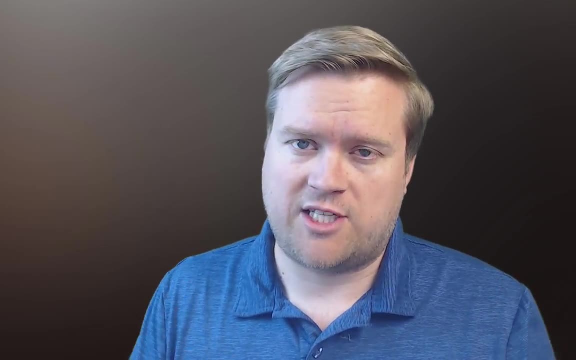 different languages. It feels like this is a much more international component framework, if that makes sense, rather than some of the more US-based ones. So if that is important to you, you may want to definitely check out Element UI. So make sure you stay all the way to the end and learn all. 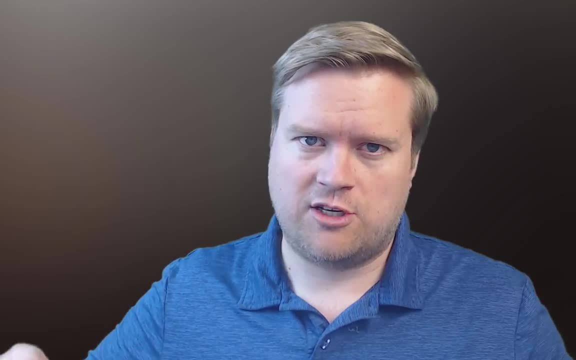 about it. Oh yeah, And by the way, if you like these types of videos, make sure you smash that like button. Don't break your keyboard, but smash it. Hit that thumbs up. And if you don't like it, 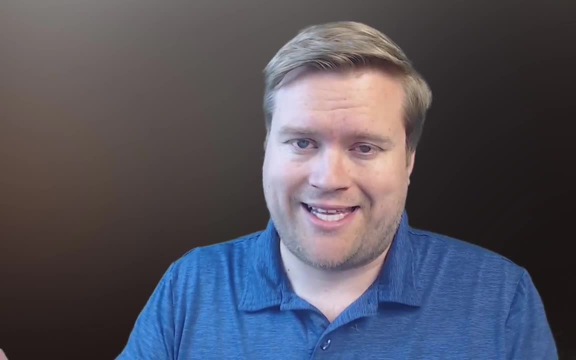 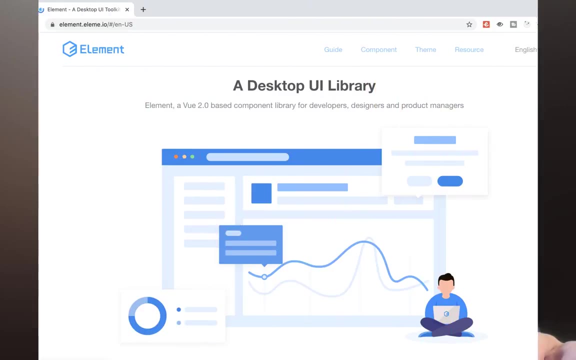 hit the thumbs down, I'm okay. either way, I really appreciate your feedback and leave a comment below letting me know what UI framework you use. So we're going to jump into the screencast. Let's go, All right. So I already. 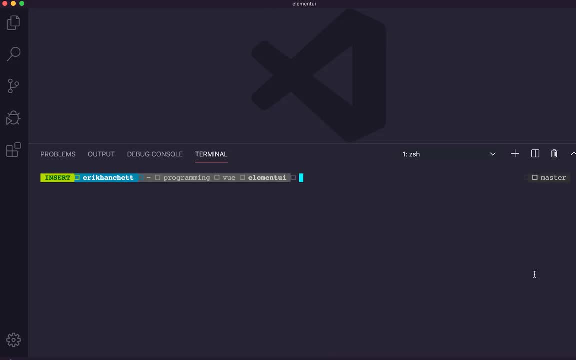 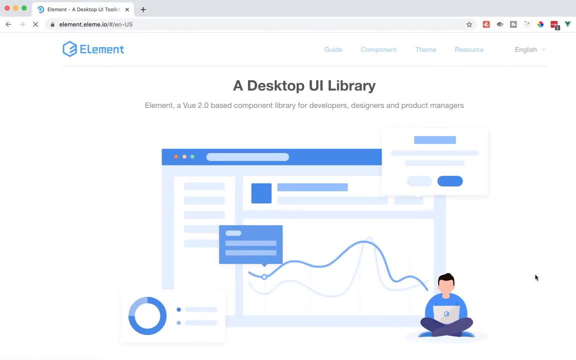 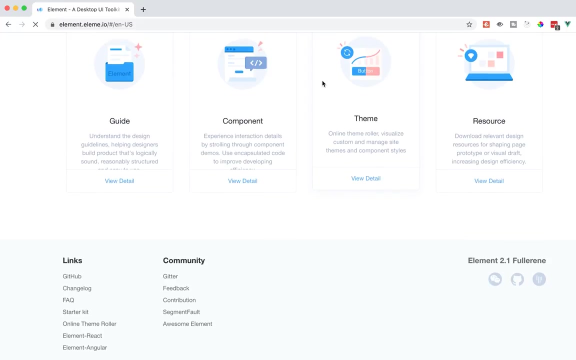 have an app that I created, which I'm going to go ahead and close- that I don't have. I haven't actually installed Element UI, so I just want to kind of give you an overview of it first. So, as the name suggests, it's a desktop UI library. It's pretty well done. The guides, components. 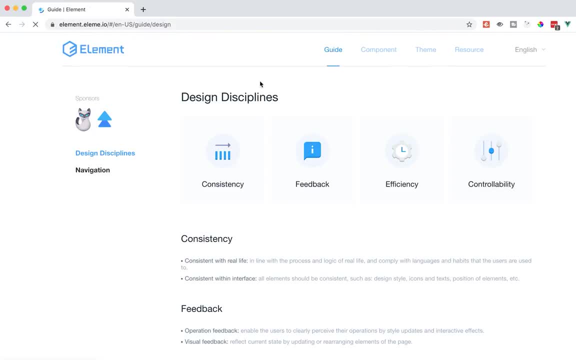 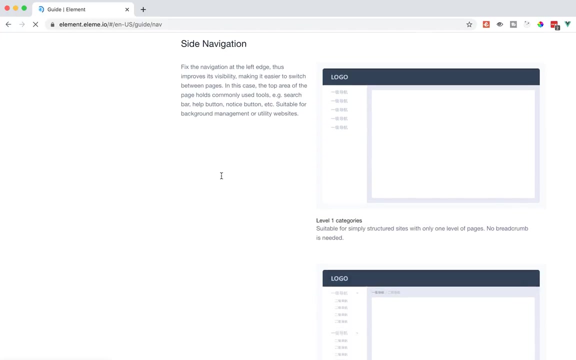 themes. it has a lot of resources for it. So let's take a look at the guide first. So they call it. they say it has lots of consistency, feedback, efficiency and controllability. That's the design principles of it. It also has a lot of different navigation. You can looks like you can do tab navigation. 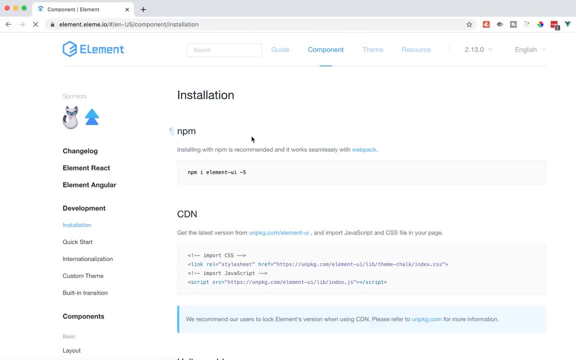 side navigation Very interesting. I think the best part of Element UI is the amount of components it has. I think it has 86 different components, which is quite a bit. I also want to say before I get in that it feels like Element has a lot of international. 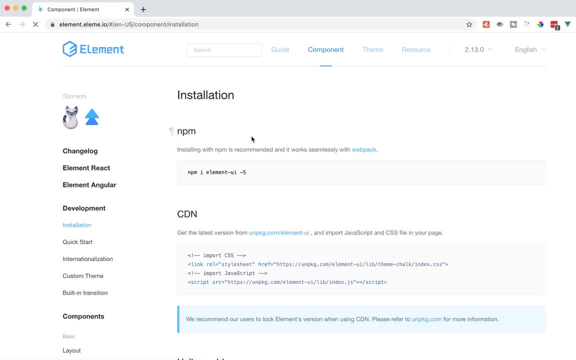 contributors. So I'm here in the United States, but it looks like it has a really big presence overseas, in China and other parts of the world, So that's great, That's awesome. So if that's a concern of yours- that you want a UI library, maybe a little bit more international, this is 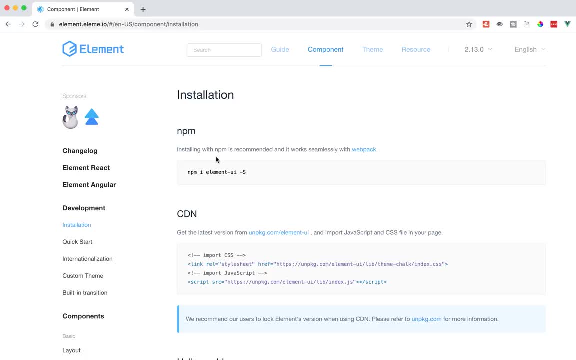 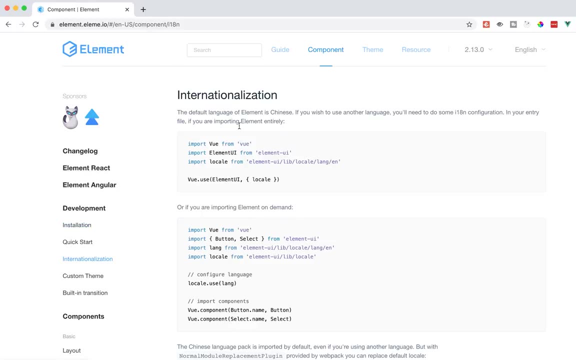 definitely the one for you. Not saying that the other libraries aren't, but that's what I kind of feel about this one. I mean internationalization is one of the key points right at the beginning, because it has a lot of. it looks like you can change the default language. 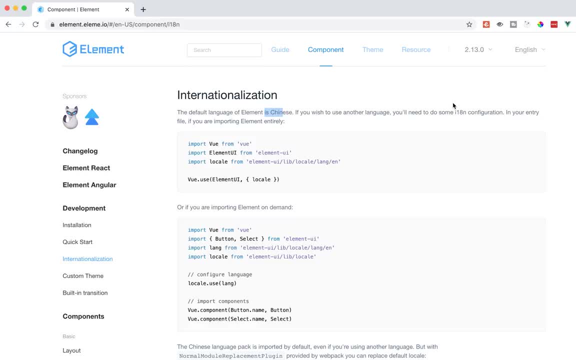 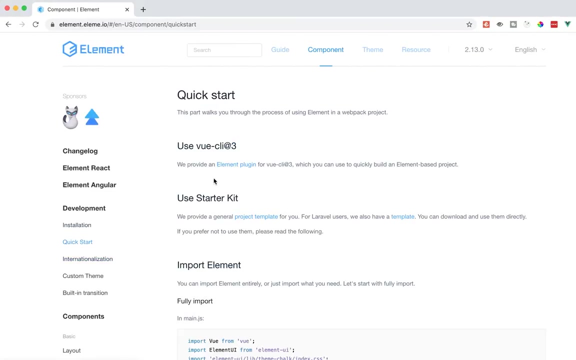 of Element as Chinese. So if you want to do another language, you'll need to do some configuration on it, which is that's fine. I know Vuetify and others. I think the default language is English. So, to get started, there's a couple of ways and I prefer the one using the plugin system. So if you 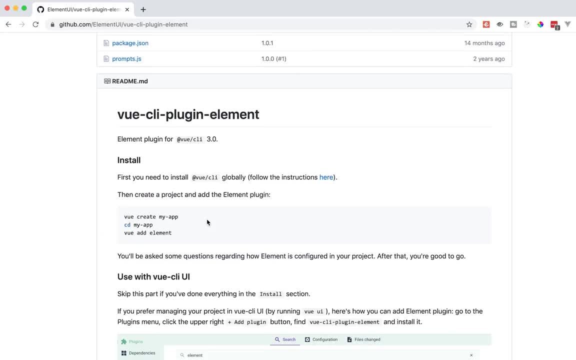 want to use the plugin system, you can use Vuetify And, by the way, these links will be in the description below. It says: all you need to do is really do this view add element. So I'm going to do that inside my app. 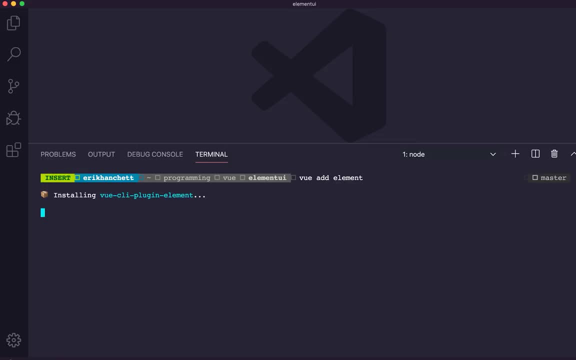 View add element, And this should go ahead and install the plugin for Element. So let's just take a moment. Okay, so it's asking us some questions here. Do we want to fully import or import on demand? Just for the sake of this demo, I'm going to just do fully import. And do you want to overwrite? 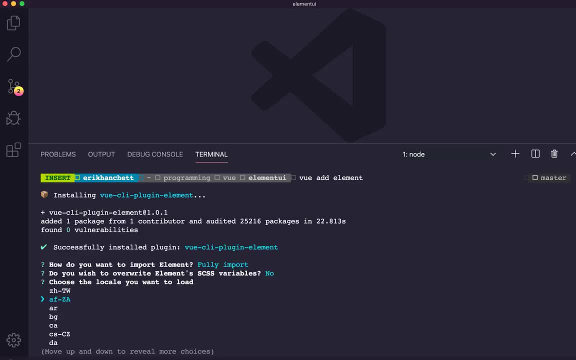 No, we're not going to overwrite anything And cool. So it asks us right from the beginning: what localization is this? And then it'll take us to the local we want. So I told you that it is very international. It has a big Chinese following. 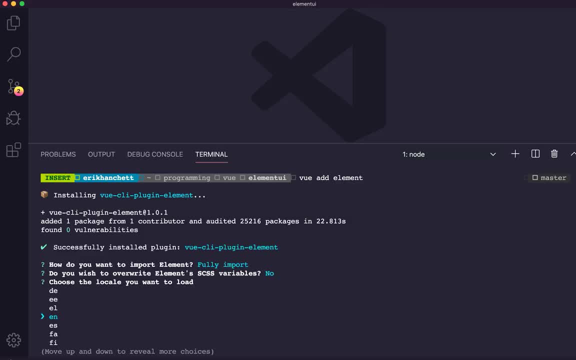 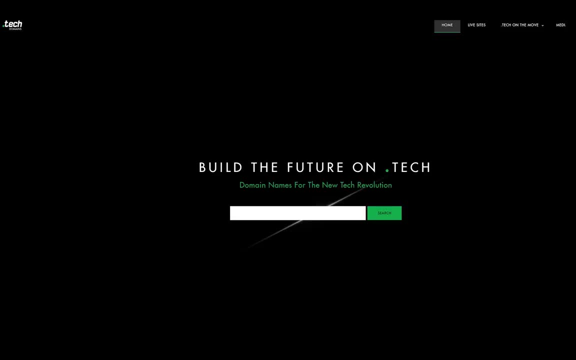 So, but we are English, so we're going to use EN for English, And this will just take a moment to install. I just want to take a moment and thank our sponsor tech Domains. Now, if you're anything like me, you probably love domain names. 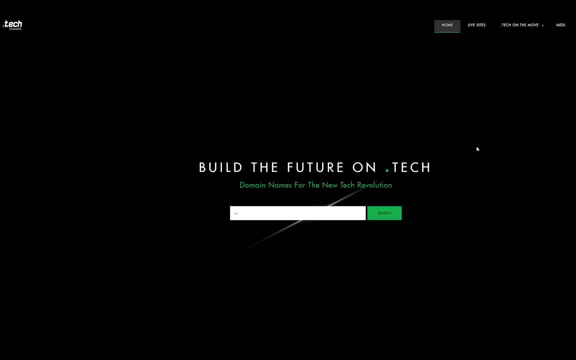 and you love to buy ones that are short and relevant but also, most importantly, available. And that's what's really cool about tech Domains. You can buy many kinds of really cool domains available and thetech domain is broad enough that you can kind of understand. 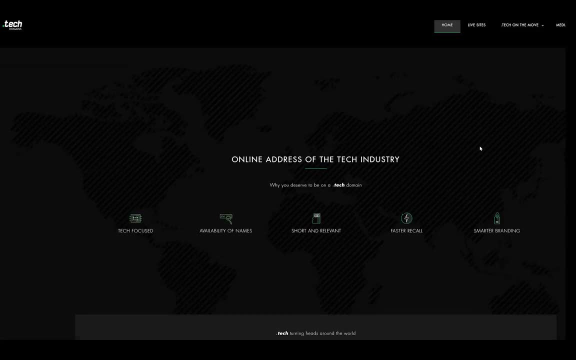 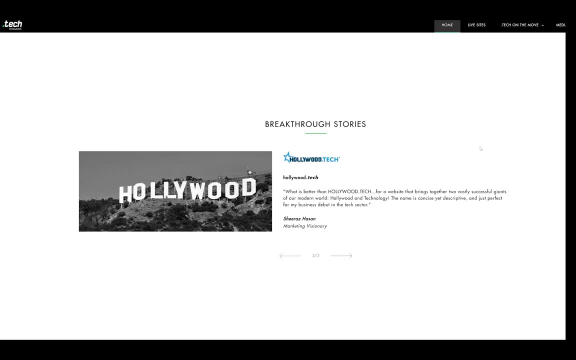 that this is technology related as well. A lot of really cool sites are using tech domains, like hollywoodtech, viacomtech, even personal sites like Austinevanstech. So if you guys are interested and you want to search for a really cool domain name, go to gotech slash Eric. 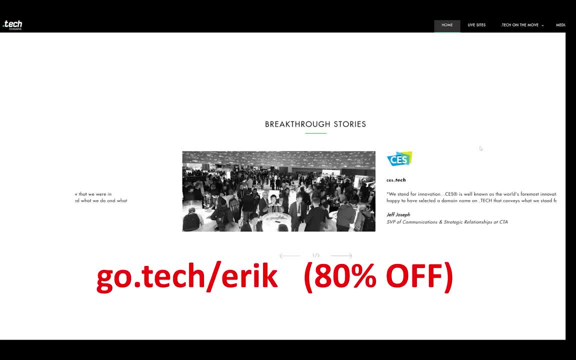 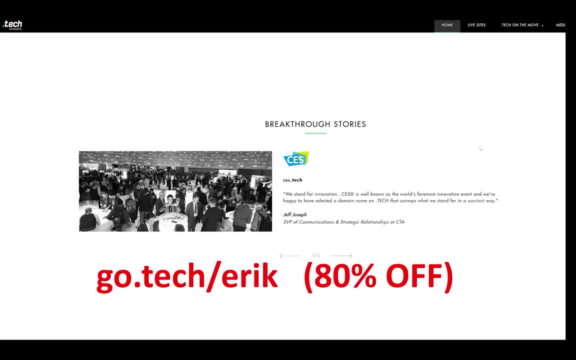 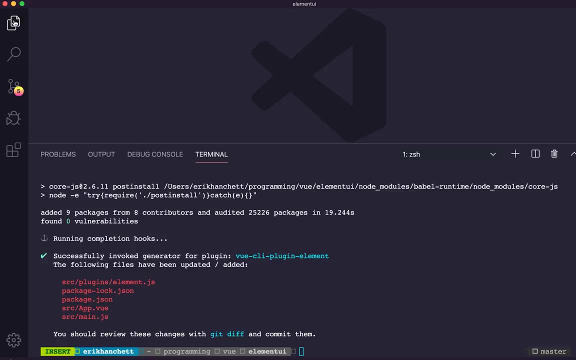 And then search for your domain name. If you end up buying it, you actually get up to eighty thousand worth of να percent off on one year and five year domains. so go to gotech slash eric and go ahead and pick up that domain name. thanks, okay, cool, and so it went ahead and set it up for us in english, so we don't. 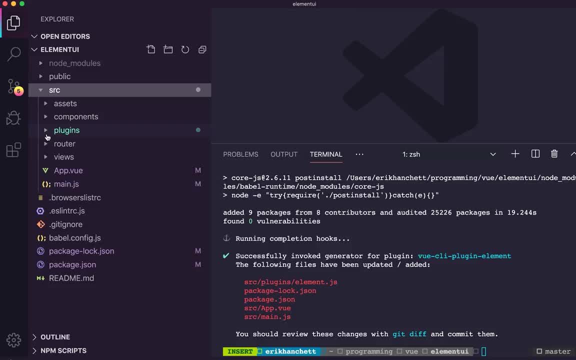 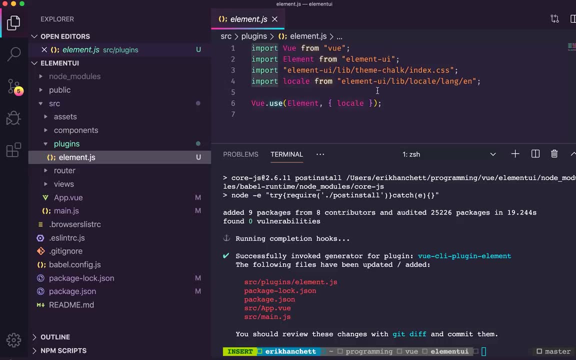 have to worry about that. so we'd see. kind of take a look at what it created. it created a plugins folder in this elementjs file. you can see this is where they put in the localization for en, for english. so that's perfect, that's what we needed. and then it made some changes to the app view file. 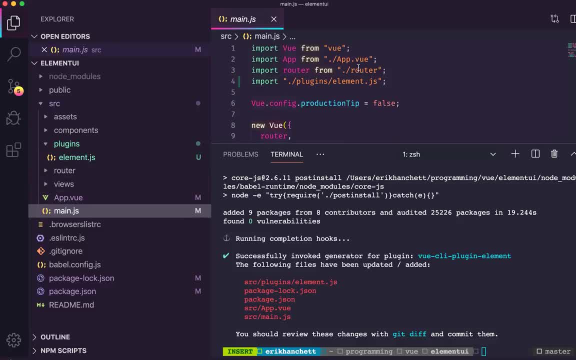 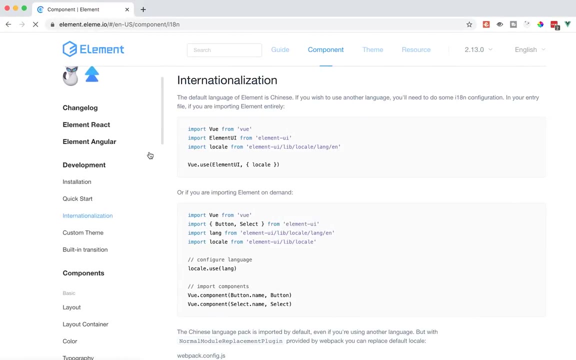 and the mainjs file. so it looks like it added in this plugins and made sure that the plugins was loaded correctly. so i think we're ready to run. go ahead and run it and see what it looks like. while this is starting up, let's take a look at what element provides us out of the box now of 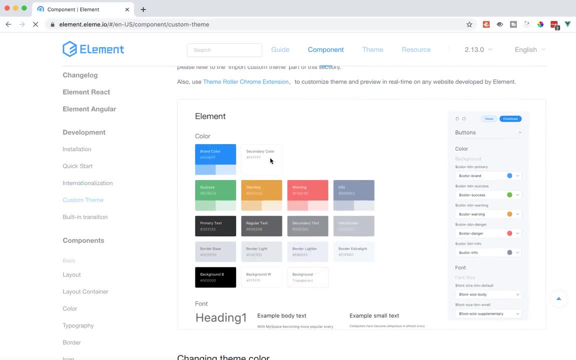 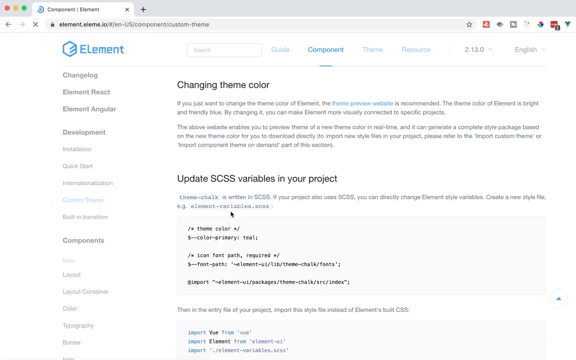 course, we can always customize everything. we can customize our default color scheme. if we wanted to, you can overwrite the element variablesscss file or create a new style file called this elementjs file, and then you can go ahead and pick up the elementscss file and then you can. 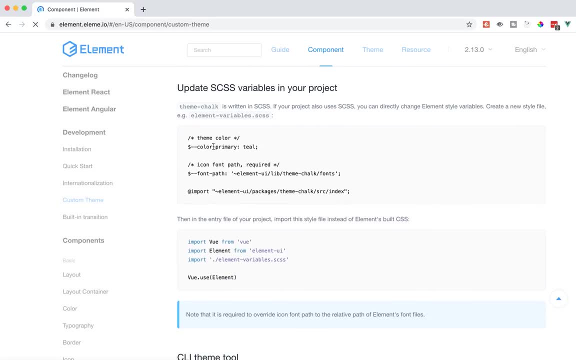 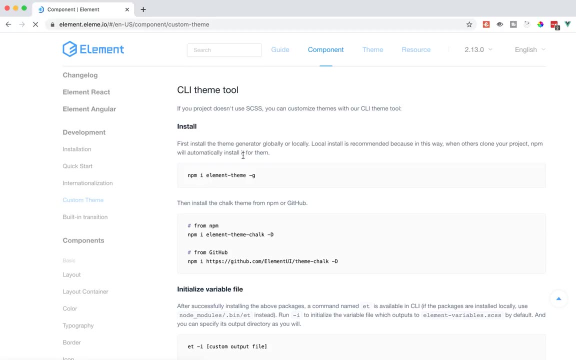 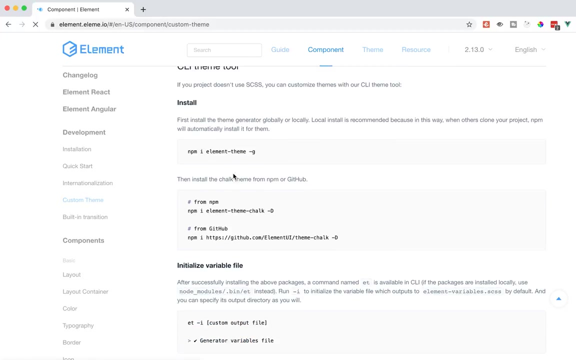 put in your own file your own colors if you want. it also has you can install theming, so you can install this elementdash theme and you can have different themes, which is really neat. i wonder if they're. i'm sure if we looked closely enough we could find what all the different themes are. 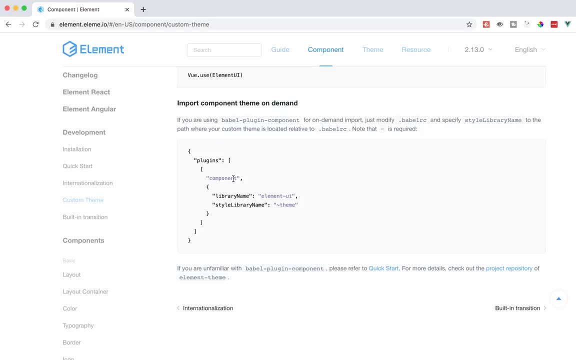 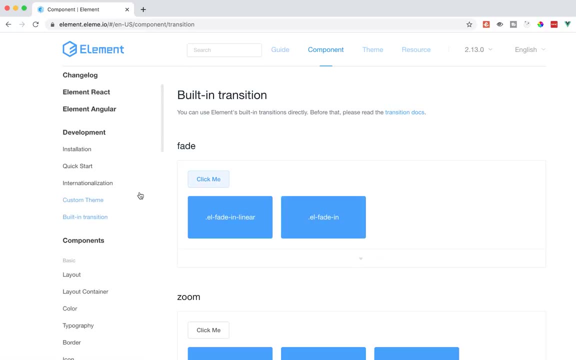 and that gives us different color schemes for it and it has some built-in transitions, which is really neat, and i'm sure if we looked closely enough we could find what all the different themes are, which is kinda neat. we can look in the transition documents. so if we look in the left, 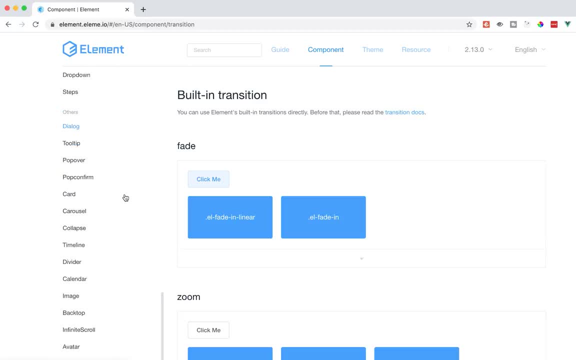 hand side here. this is all the different components. like i said, there's quite a few of them. i want to say there's over 80 of them, and so this is almost as big as is viewedify, maybe even a little bit bigger. in fact, if you go to viewedify's website, i'm going to go to viewedify. i was just looking up. 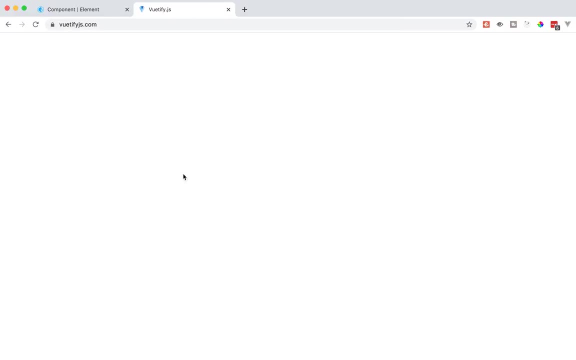 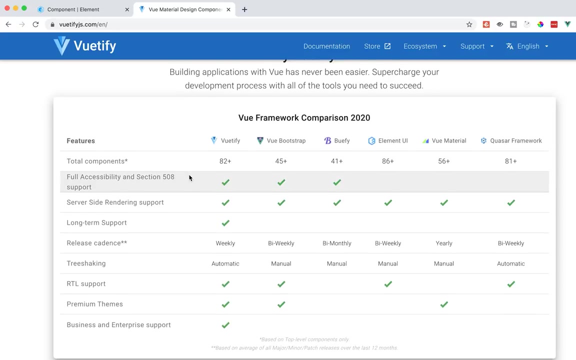 some stuff on parallax they actually have on their front page- which is really amazing that they're so- to other UI frameworks for Vue And they say that Element UI has 86, while Vue Defy only has 82. But Element UI doesn't have full accessibility. 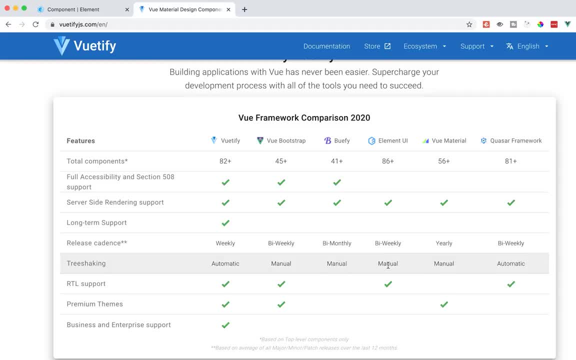 It also doesn't have long-term support and tree shaking is manual. So when we set it up we actually did a full import, so I think we have everything. So it sounds like we probably if we were using this in production. 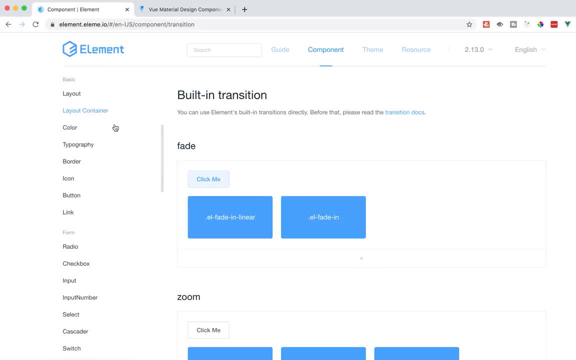 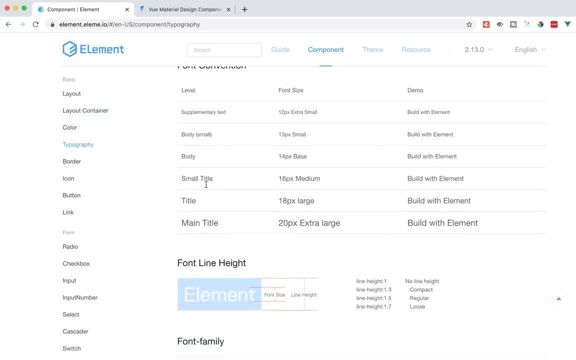 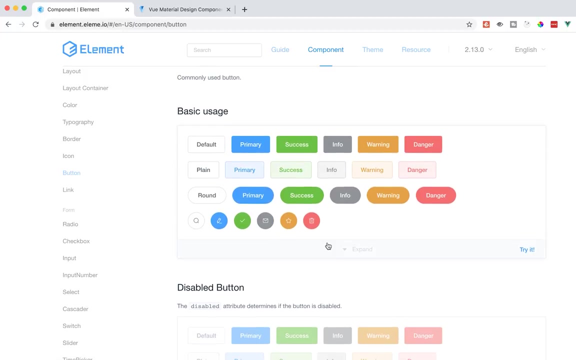 we'd wanna just import the ones that we want. You know, as for this there's, as for the components, there's just tons. obviously, typography- having Chinese support's really important- has borders buttons. I think buttons are a good example of just what you can do. 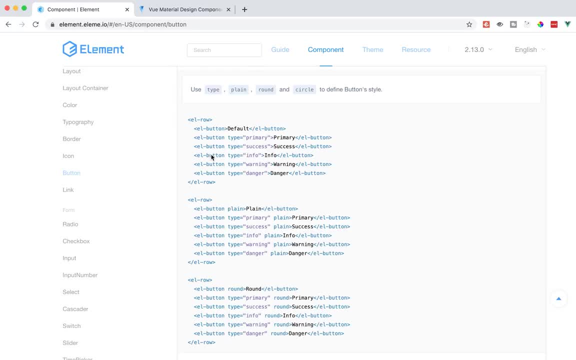 So I'm gonna expand this And you can see you use this el-row and that's the column layout. Let's see, I think there's a whole section on the columns. Ah, there we are. Let's see here if we look. 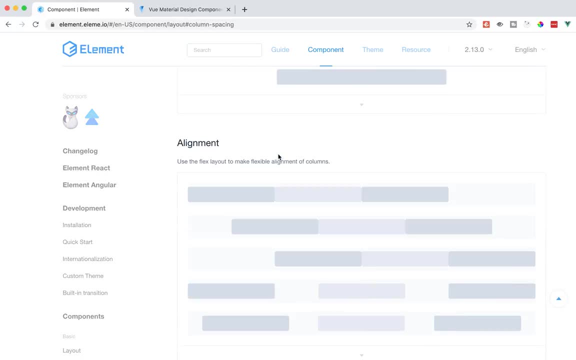 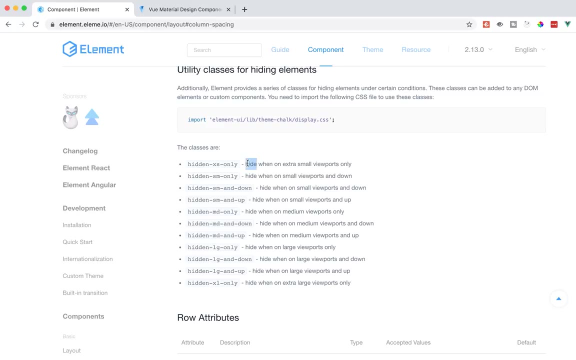 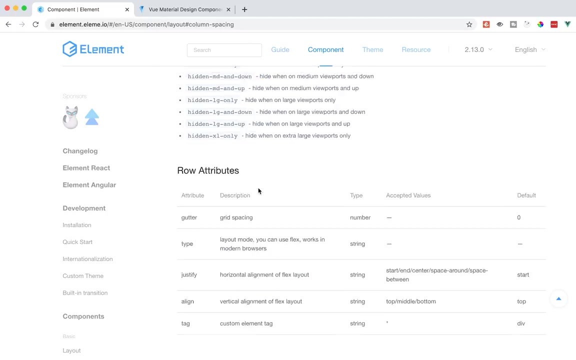 Column layout. column spacing: Yeah, you can kinda see it has similar to this 12-column layout that you see in a lot of this. other frameworks You can also use. You can have different viewports by assigning different kind of utility classes. 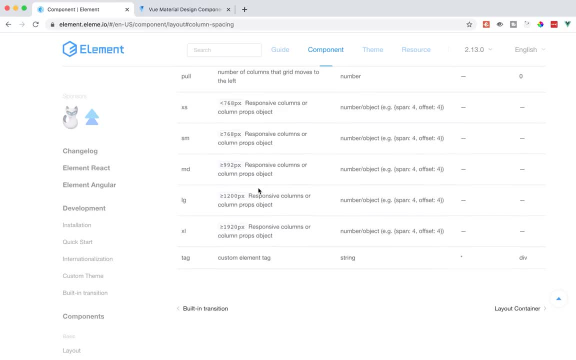 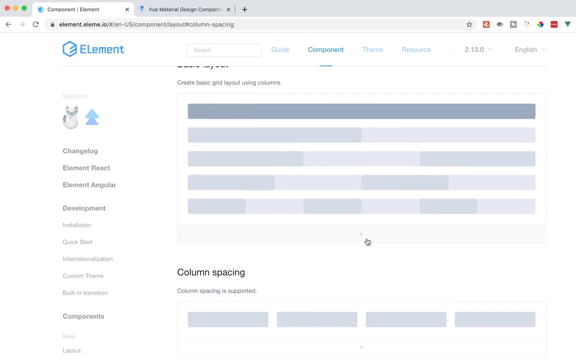 it looks like. So that way it doesn't show up in different different sizes to add them as attributes inside your EL columns. So here's like the basic layout. if you expand it here You could do this EL dash row and then you put the span. 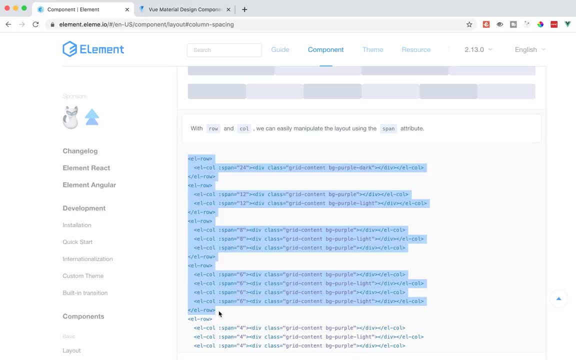 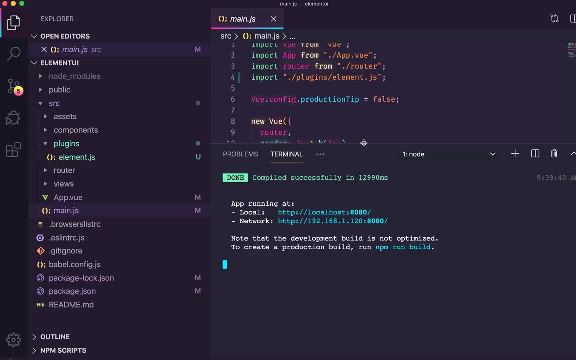 So let's see if this will work. I'm going to copy and paste this first before we go into our buttons, So we don't need that many of them to make sure our app works. OK, so we are running right now. By the way, let's open it up in localhost 8080 and take a look. 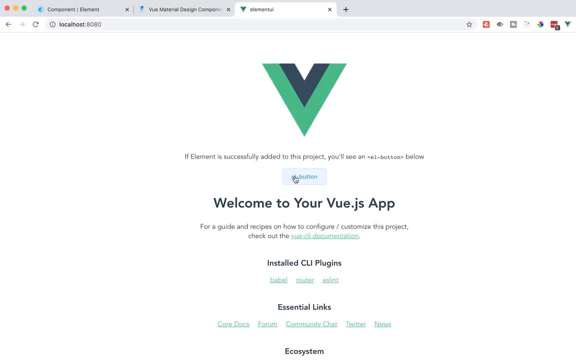 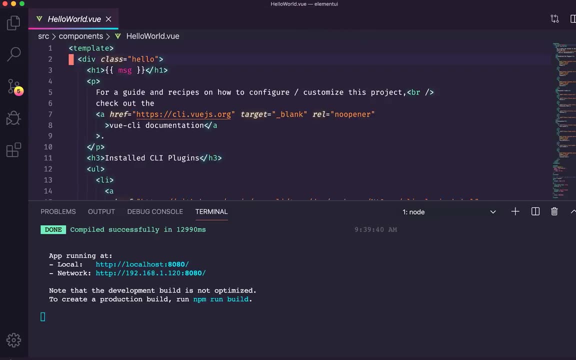 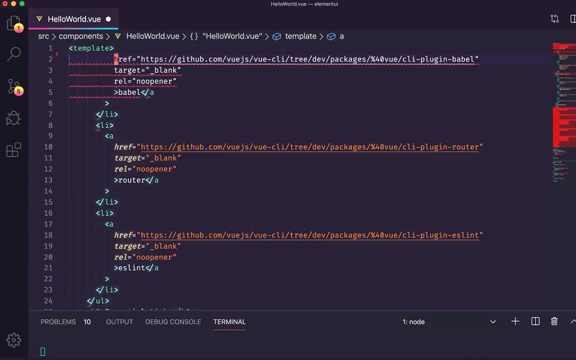 Cool. So here's- oh, it even has an EL button right here. Element is successfully added to this project. So we're going to be kind of lazy and just edit the Hello World app here, And I'm going to make this a little smaller. 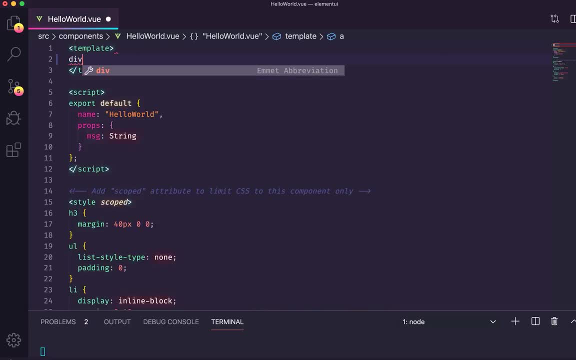 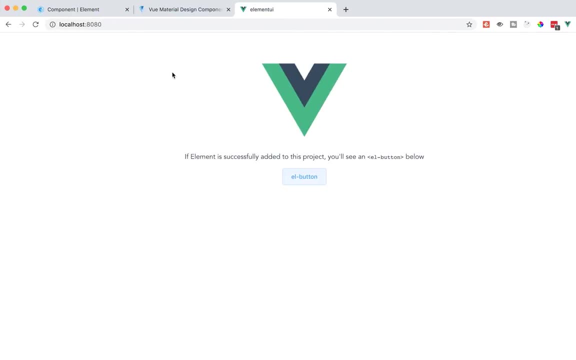 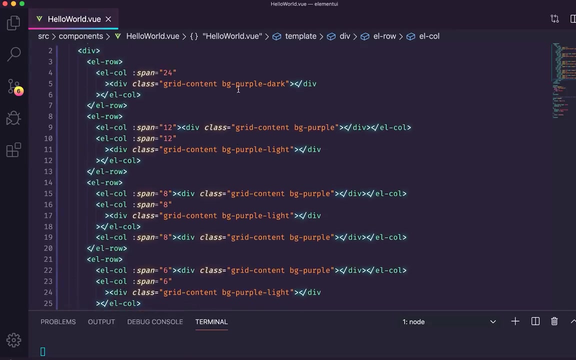 So this will just take a moment. Let's see here- And I have a div tag in here- Here's our EL rows. OK, they're all nicely formatted, Cool. So element successfully added. Let's see if. do we have any data in here. 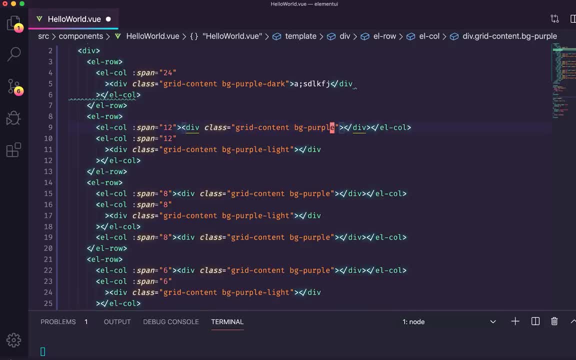 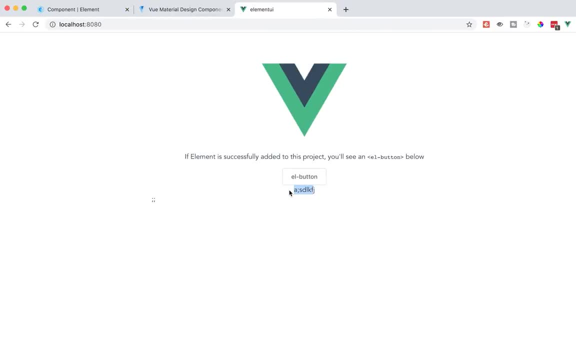 I guess we have to actually type something in some of these columns. Let's see if we save it. All right. so here's that. Let's try the buttons to see if it's working. I'm not sure if it is, Oops. 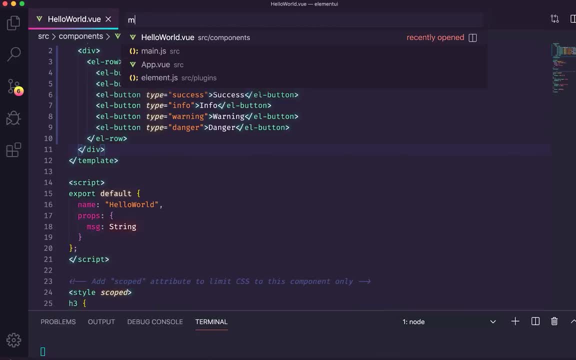 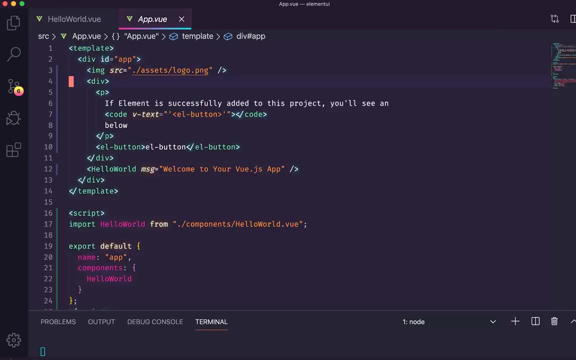 OK, cool. So, yep, Yep, these are working correctly. Let's go into. let's clean this up a little bit. We'll go into our main. well, let's go to our app view file And you can see here that it has this paragraph tag: 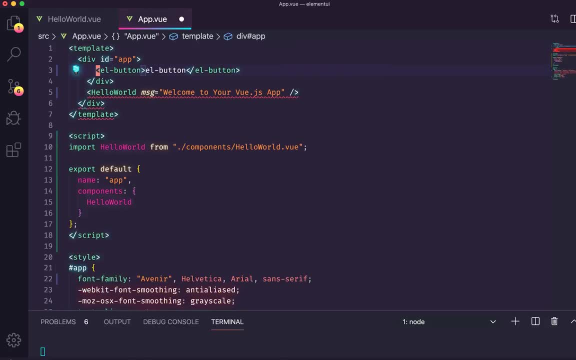 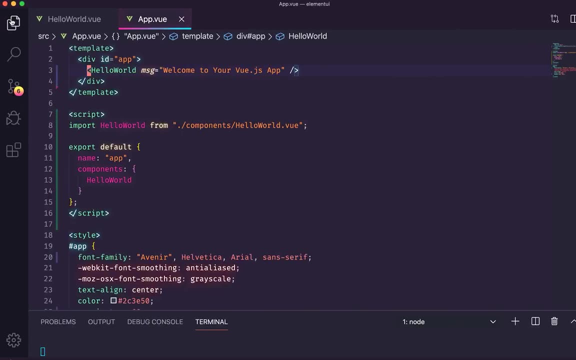 Delete the image And delete the EL button here. Cool, so now I have our primary success. I have all our buttons showing up, So we go back to our Hello World. You can see, we just put a type in and then this makes the different. 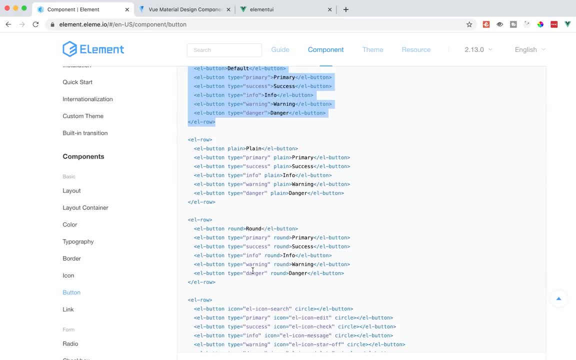 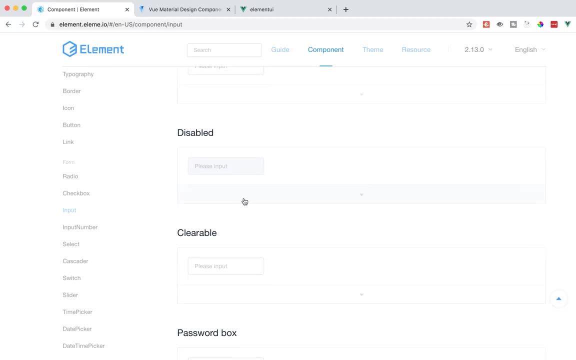 Cool. So this is just one of our colors, which is nice. What else can we do here? Let's take a look at input boxes. I think this is a pretty normal. I mean, these are pretty generic looking input boxes, But you can also nice thing about the documentation. 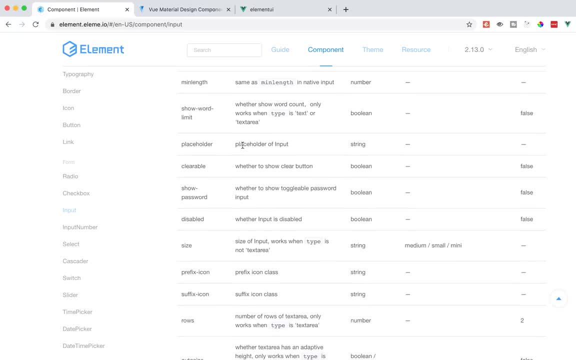 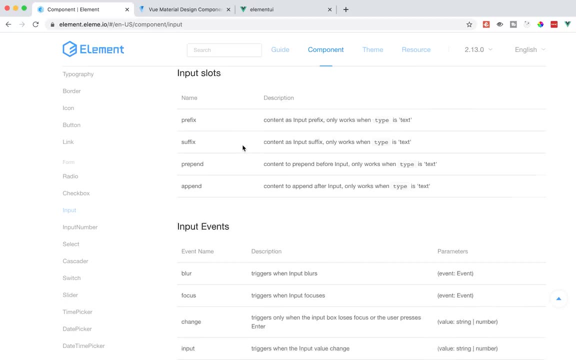 it tells you there's a ton of attributes you can put on it: Min, max length, clearable, disabled rows, auto resize, read only, And then it obviously hooks up to. you can have different slots on there. input. 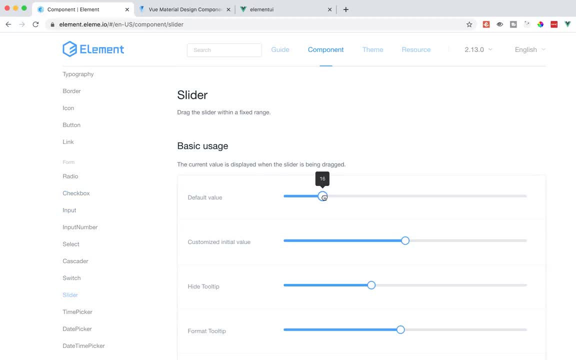 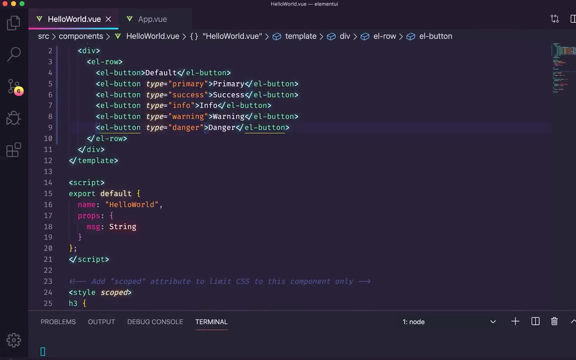 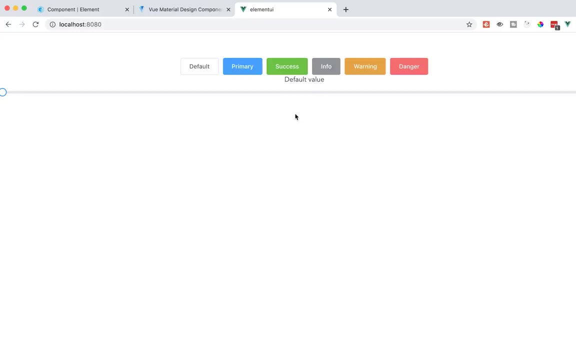 elements. Let's try a slider instead. It's kind of neat, So we can always click Expand here, And I'm going to grab one and add it to our app. So we added a slider. See if it shows up. There it is. 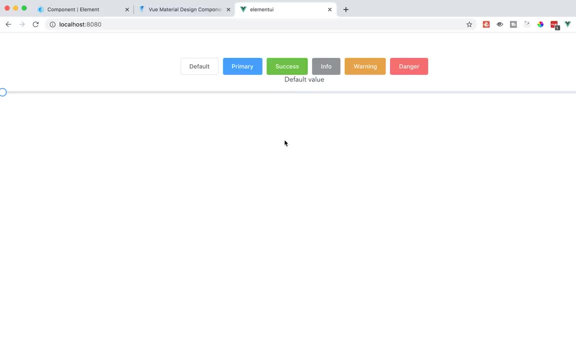 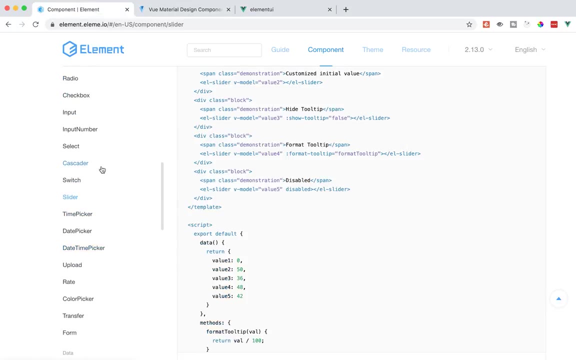 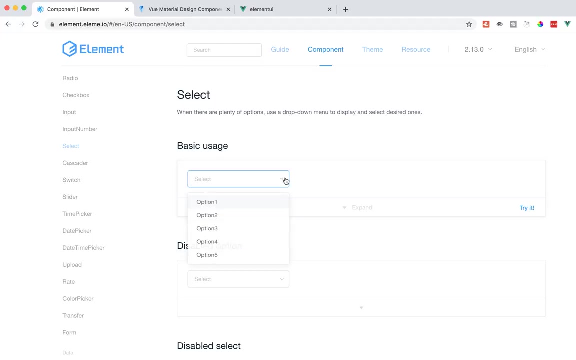 Here's our slider. Kind of works. default, Looks pretty easy, Nice, Let's try. let's see The Select drop down. All right, It kind of has like a little bit of an animation to it. Makes it nice. So here is the select. 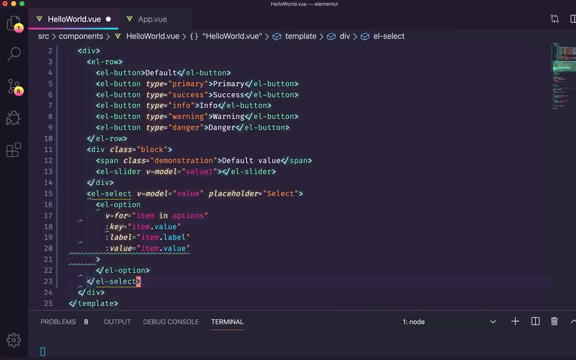 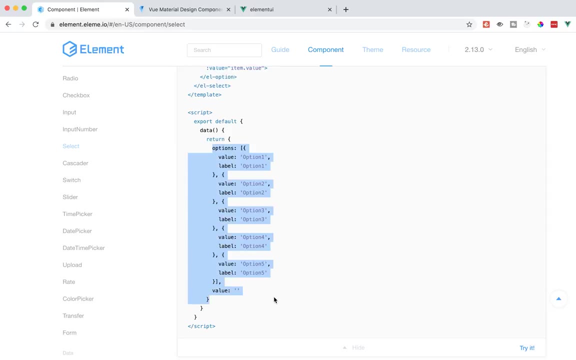 Let's just try that out. And now I have to actually add an options with a key of value. So let me see, here I'm going to have to add some stuff. Oh, here it is, Let me add this return. And then I'm going to do this. 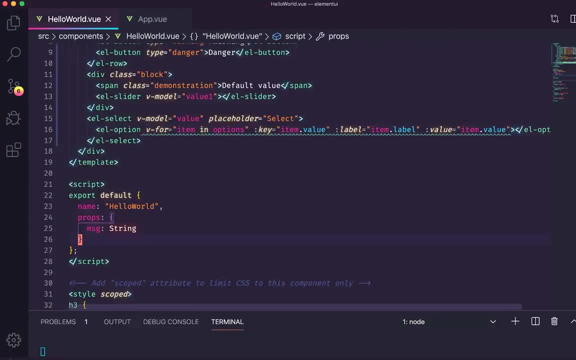 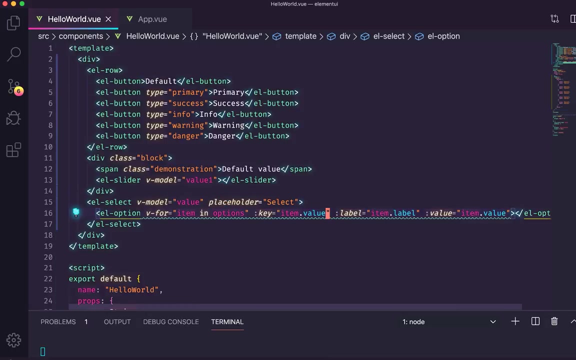 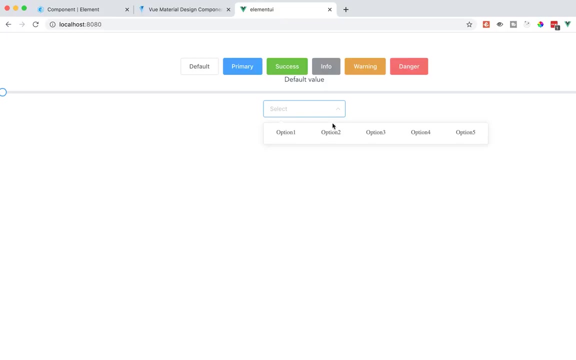 OK, OK, OK, this options. so I'm gonna create. we'll just go ahead and copy and paste it all from the data object on. okay, now we have a data object and I'll just fix this prettier error. okay, there it is. let's take a look. cool, here's our select drop-down. looks like it defaults. 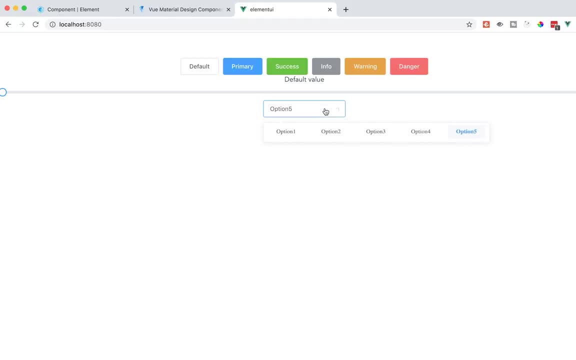 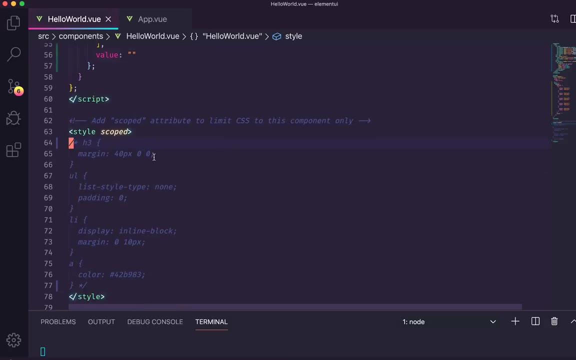 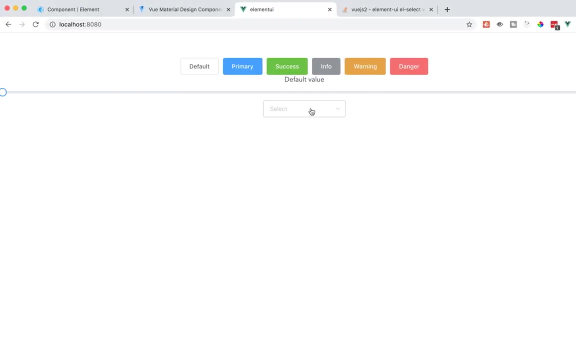 to not being on top of each other, which is interesting. I wonder if there's a setting for that. oops, actually, I found out the issue. some of the CSS code here was doing an inline block and it was causing it to show incorrectly, so that's why it showed horizontally and so vertically. so now here it is. so now it's. 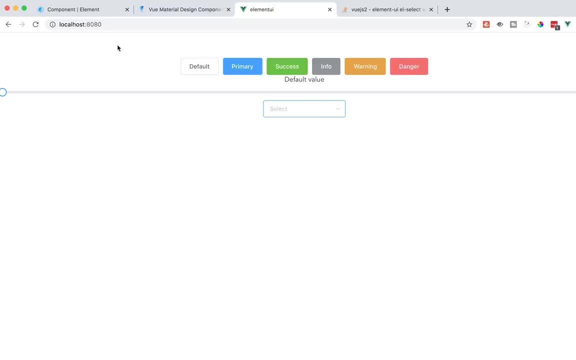 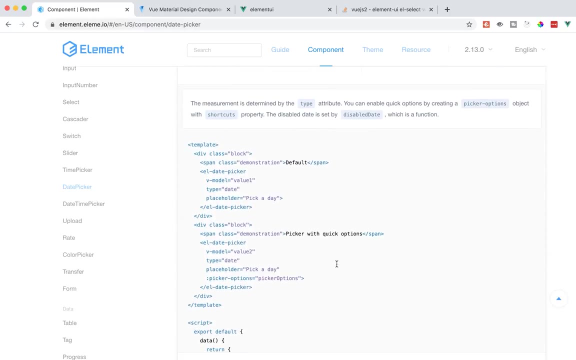 working as it's supposed to, with a little bit of an animation, one which makes it look nice. maybe we'll look at one more this date. picker looks kind of interesting, but I bet it's not going to be as interesting as it should be, but I bet it's pretty involved, but it looks like that's not too bad. you can in the. 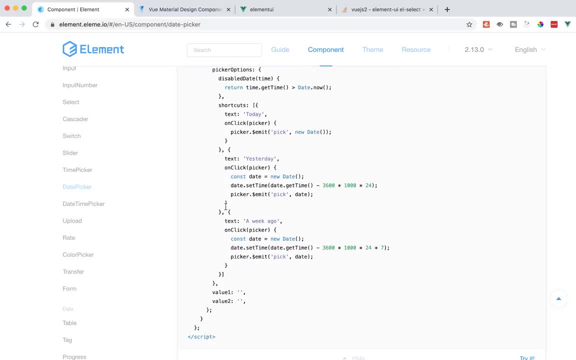 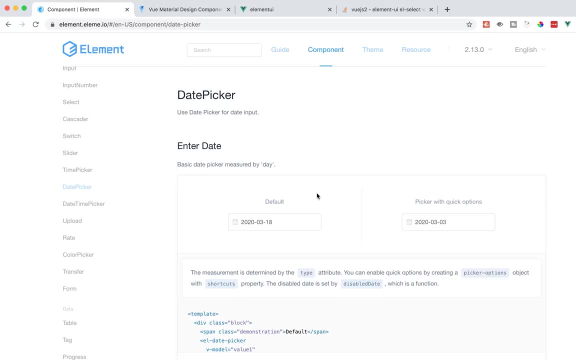 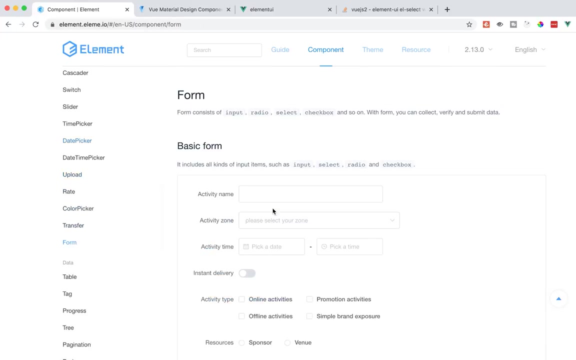 return options. you do the picker option, the shortcuts. yeah, it's pretty long but I'll just show it to you guys through. here. there's this full calendar option. you can select different dates you can have. you can have a minimum and maximum date, which is kind of neat. let's take a look at forms. so lots of different form. 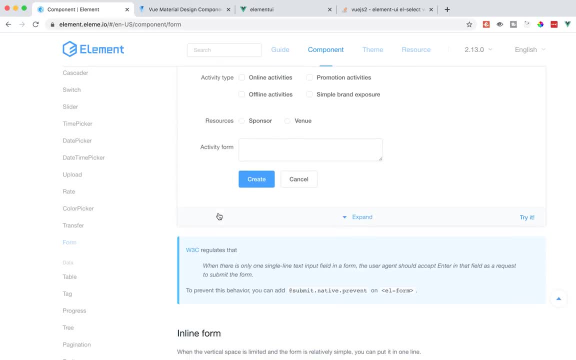 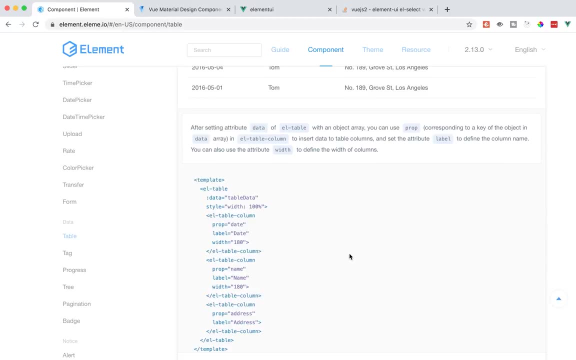 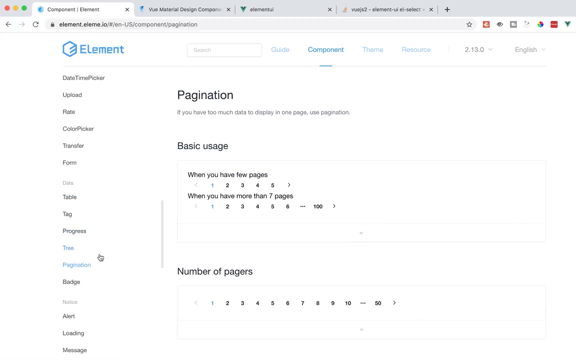 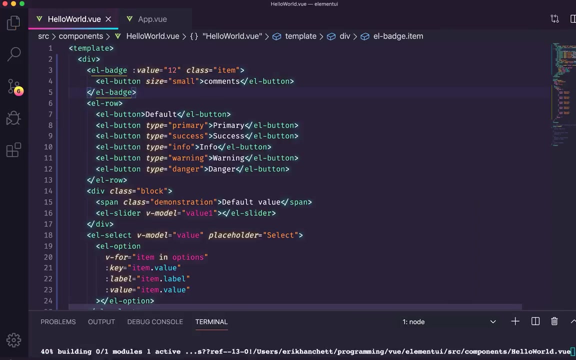 options here. inline forms has whole tables inside here which you just use el dash table and you can actually add the table. data has pagination, has badges. how does these badges work? it looks like these are pretty easy. let's, let's add a badge to our app here. add it to the top. cool, here's our little.